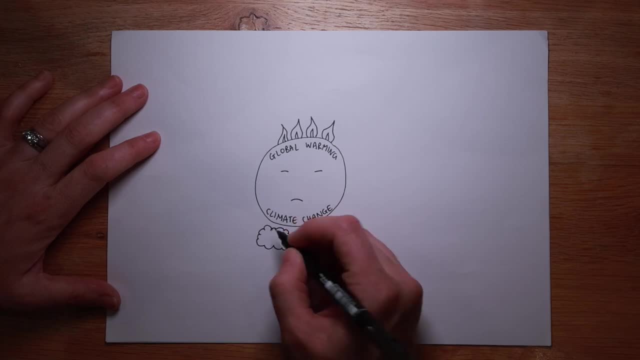 but climate change is things like sort of extreme weather events happening a bit more. so we're seeing kind of more storms. So if you want to put storm cloud in, we're seeing basically the frequency and the intensity of storms going up. So more storms. 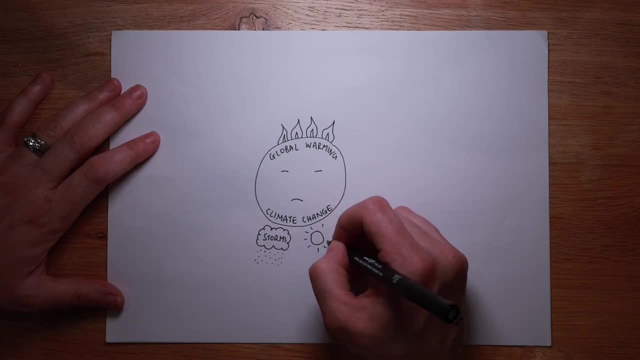 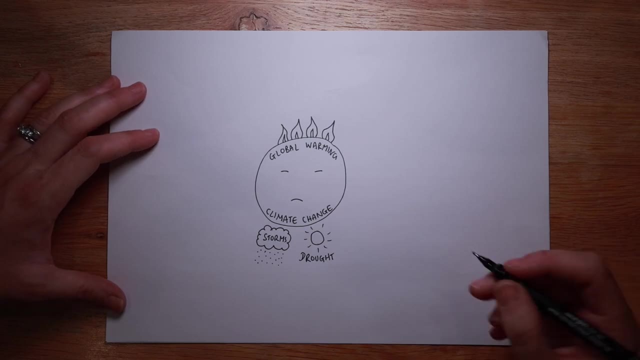 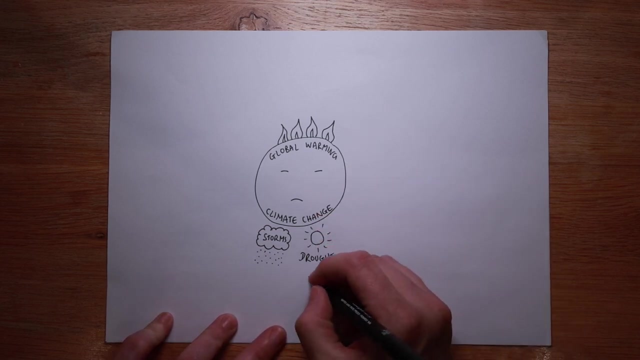 likewise, I'll draw a sun here. We're also seeing more droughts. A drought is when there is a period of very dry weather for weeks, sometimes months in some places, And then, leading on from that, we can often find these are trees. 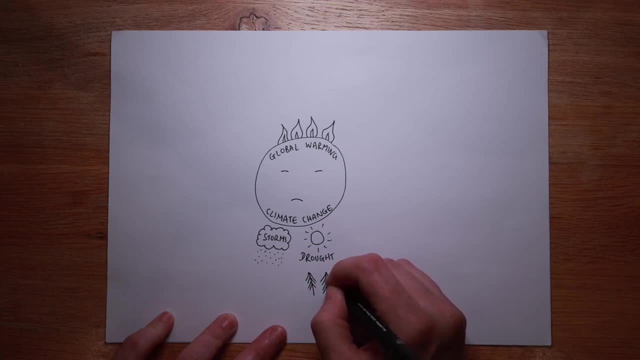 wildfires or bushfires and some forest fires they're sometimes called. Again, I'm going to draw one of my flames in there. The flames can reach the top of the trees in fact, but I'm just going to draw them like that for now. So the incidence of wildfires 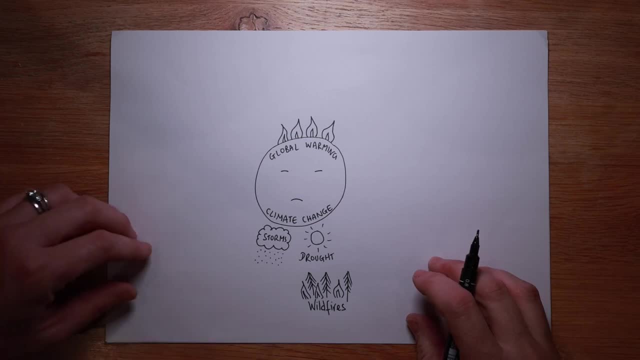 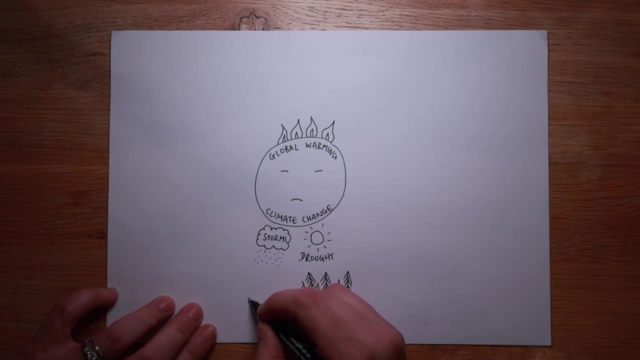 the amount of them, the severity of them, is going up. And all of this if we're thinking about climate, we think about weather, yes, but we're also thinking about temperature, And that has gone up quite drastically. So we're going to write in there: temperature increase. 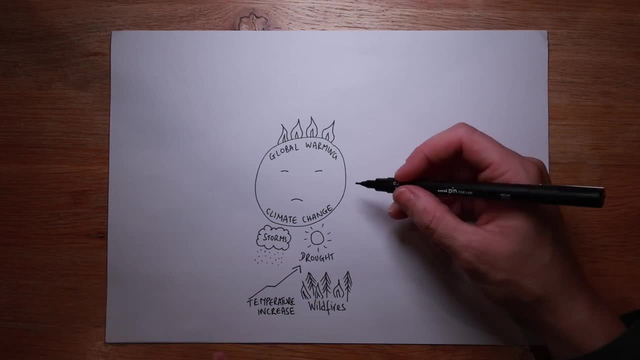 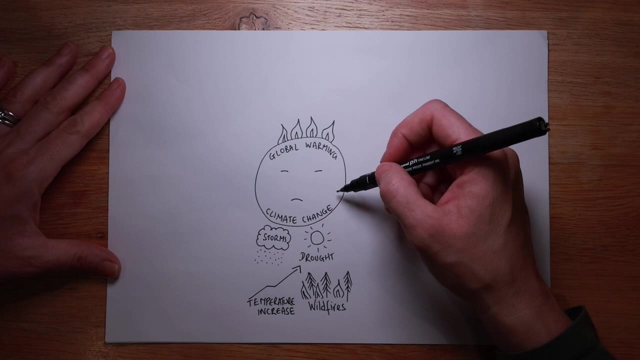 Okay. so we know. we know what the problem is. we know what global warming is we've done. I've got another infographic on the greenhouse effect and what's causing that. Today's infographic is really looking at what we can do about it. So there are two factors here. 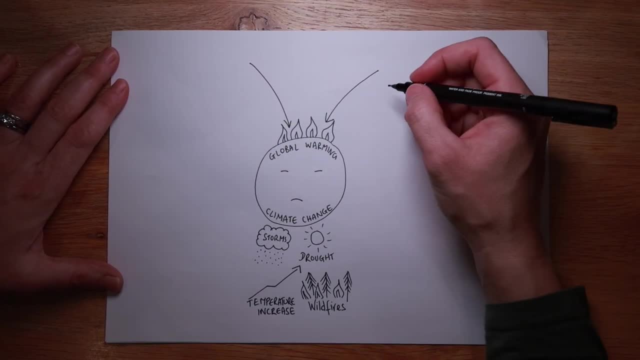 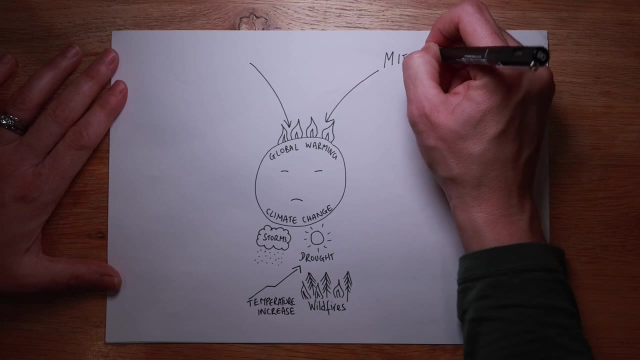 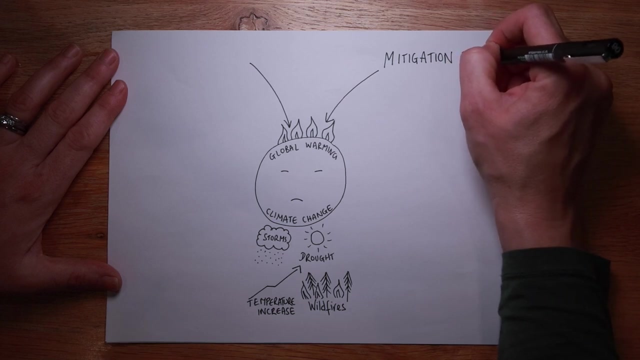 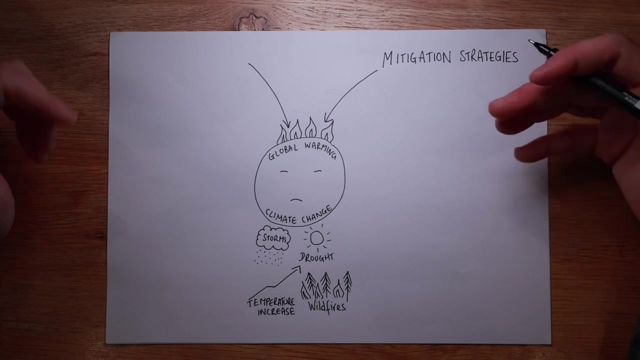 things that we're going to discuss, if you draw two big arrows. the first one is something called mitigation. now, mitigation, mitigation- there we go. mitigation strategies: these are things that essentially are there to try and reduce both global warming and climate change. they are not ways that we're adapting to it, but actually ways to slow it down. we now know that we. 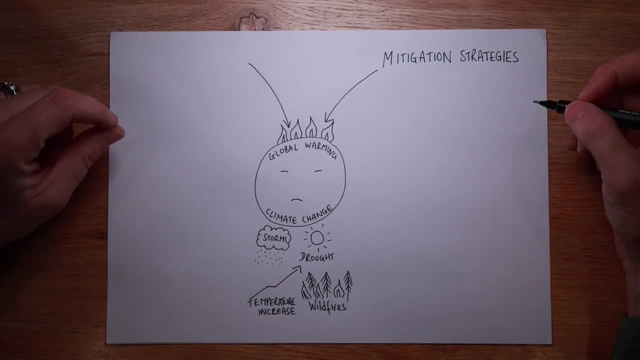 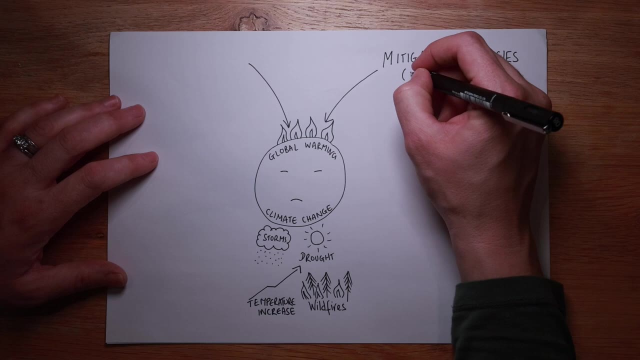 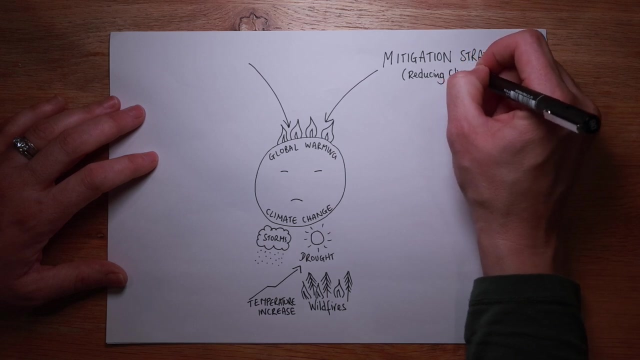 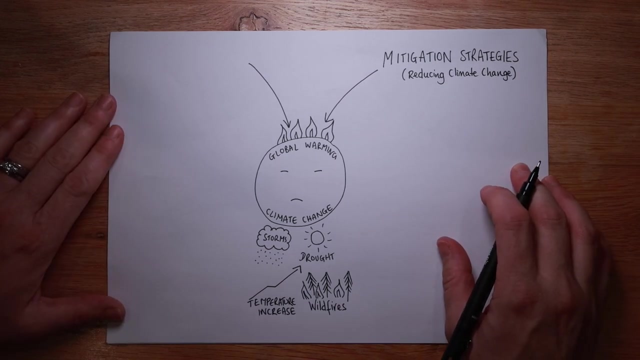 can't stop it, unfortunately, but we can slow it down and we can do a lot to kind of reduce those effects. so if you want to just put in brackets, it's about reducing kind of climate change, okay and and stopping it being so bad or as bad as it's predicted. then on the other side we've got something called adaptation strategies. 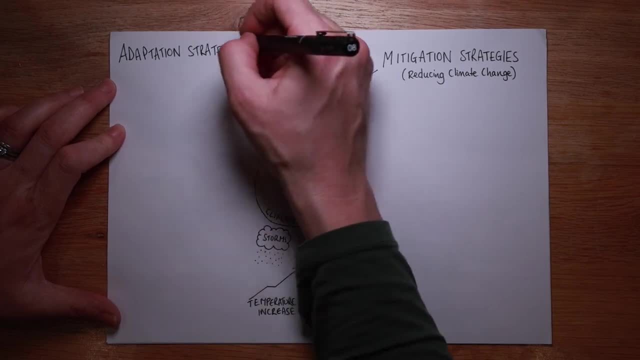 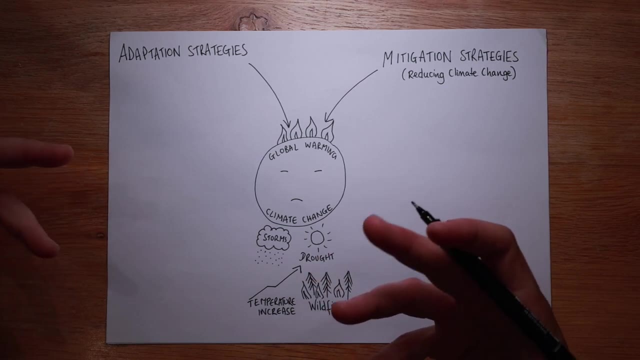 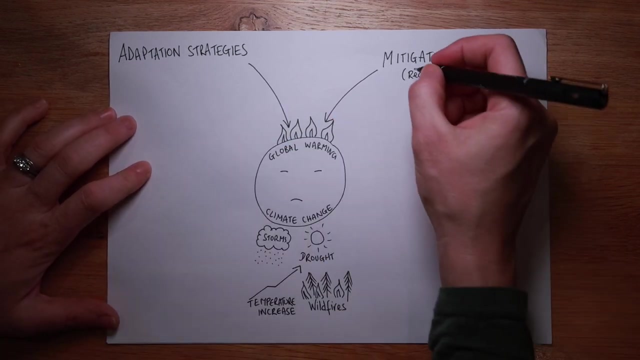 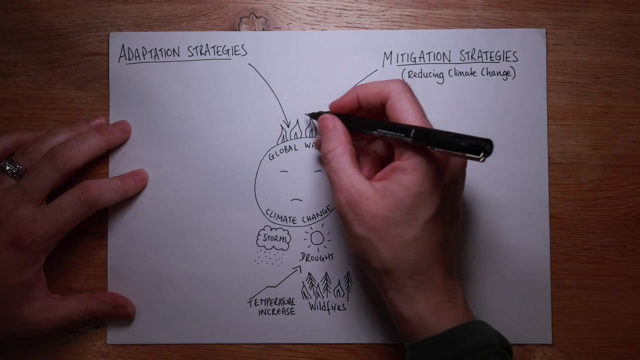 now. these don't do not try and solve the problem. these are only focused on how to reduce the impacts in the short term, to help our lifestyle, to enable us to keep food on the table, to stop homes from flooding. they are not having any impact on actually dealing. 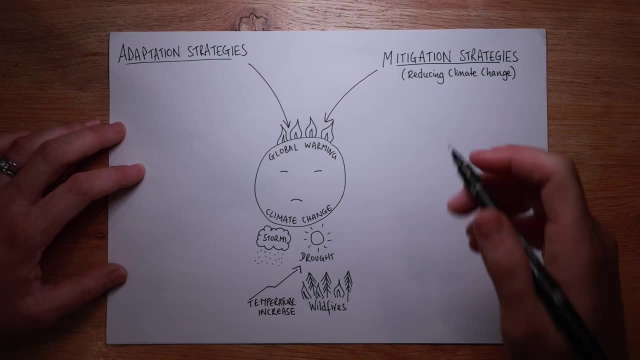 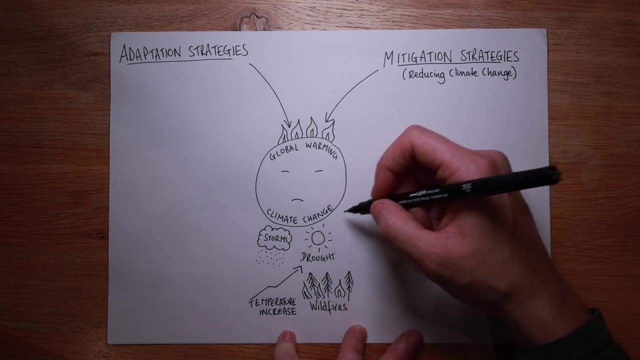 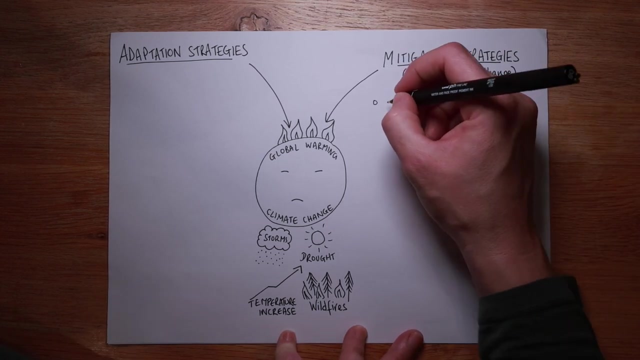 with the problem. so we're actually going to start with. where should we start? should we start with actually dealing with the problem? so we we know that global warming is caused by burning fossil fuels. that's one of the biggest problems. so the first strategy, so that, probably, first strategy. 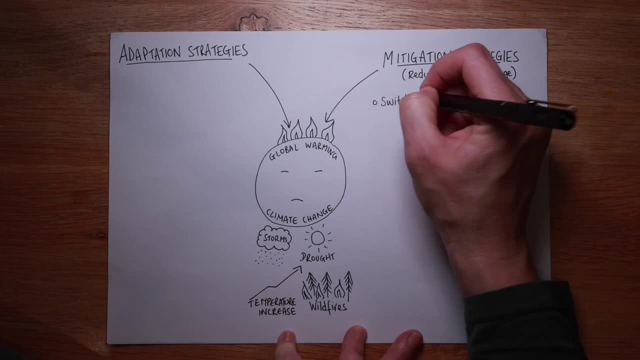 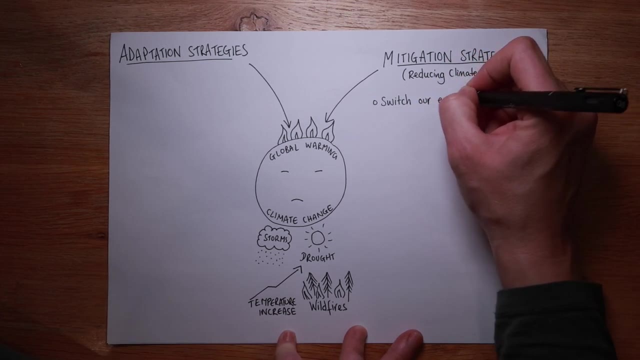 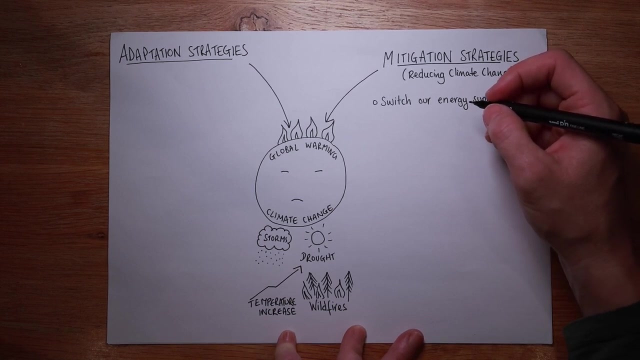 is to actually switch our reliance, our energy supply, from fossil fuels- uh, to renewables, and i've seen this happen. been teaching now 14 years and when i started out renewables- so back in 2009- uh, renewables were about five percent of our electricity and now they are well often about 40- 45 percent. so we are ought in the long run, they are. 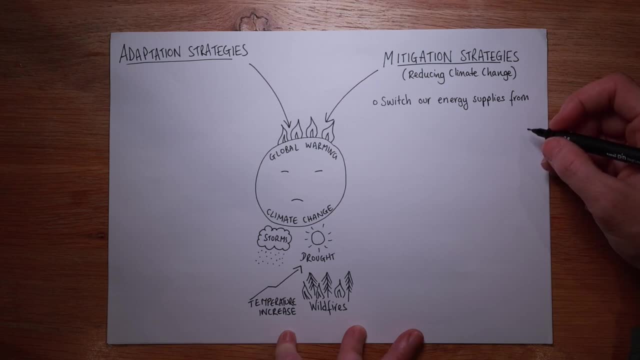 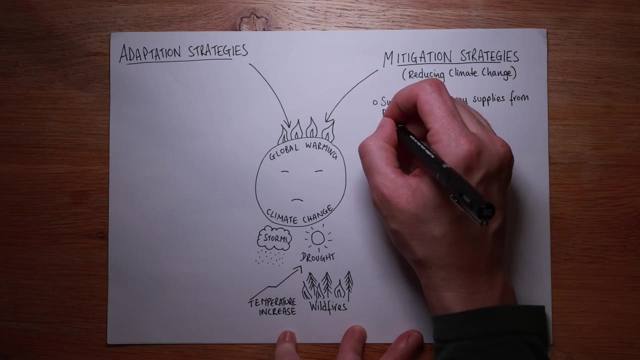 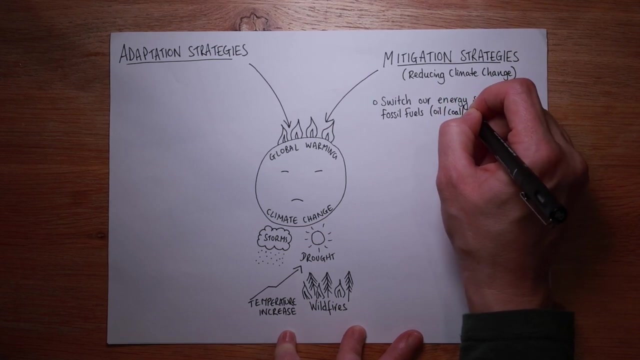 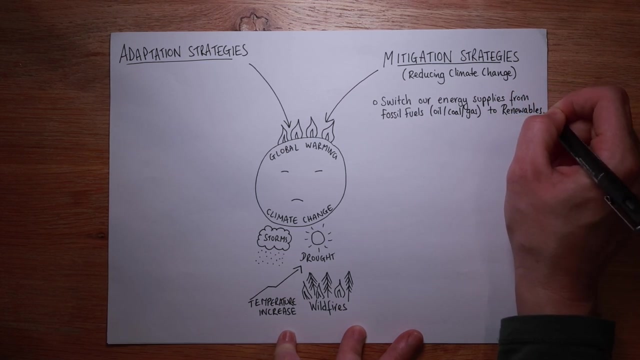 cutting open across bulk energy services. all caps- up to 35 percent of coal Smokes are cutting up those sweeping pollution rates. but we've managed to bring up more, braking these. so it's gone up hugely. so we need to switch our energy supplies from fossil fuels, which is oil, coal and gas, to renewables. now it's not enough to just 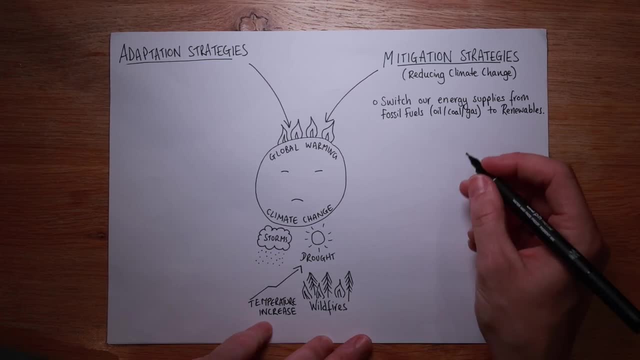 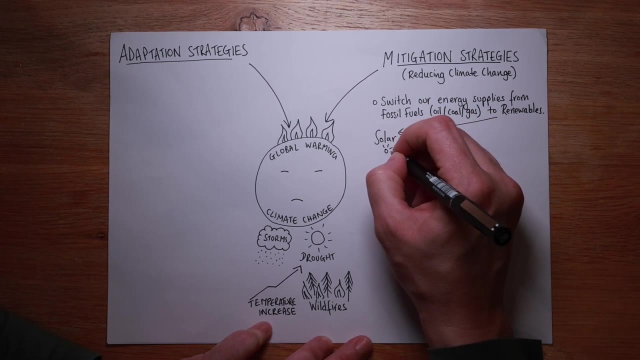 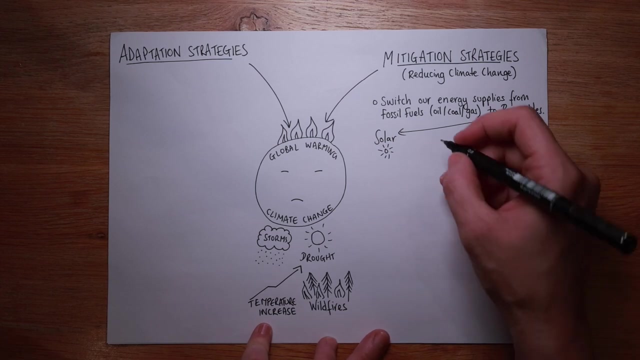 put renewables, because we AQA would expect you to talk about those renewables. so the first one is solar, which works obviously really well. in hot countries we have solar. here we have some solar farms, but it's not- um, it's not our biggest one by any means. however, wind power is huge in the UK, so I'm just 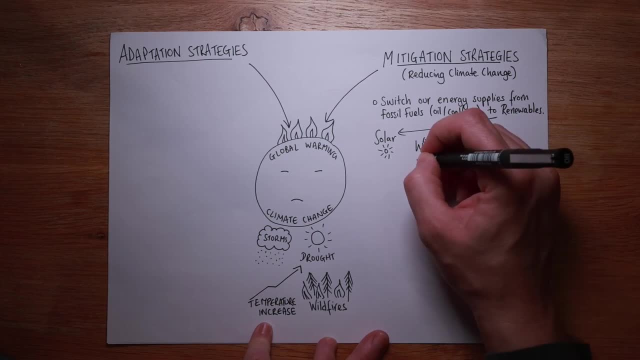 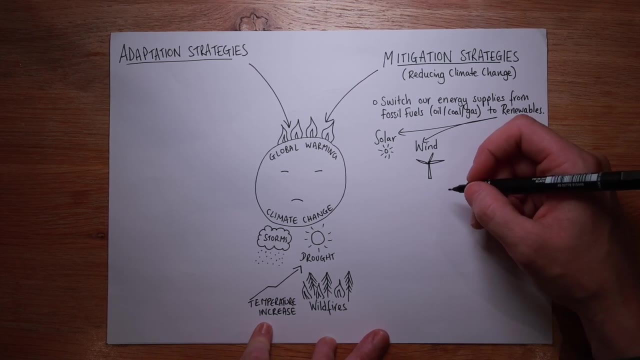 going to draw a little turbine. we have Anglia one, we have Anglia one. we have Anglia one which is a huge wind farm. and we, out off the East Coast and nearer where I teach, near Sussex, well, in Sussex we have a huge wind farm just off the coast of. 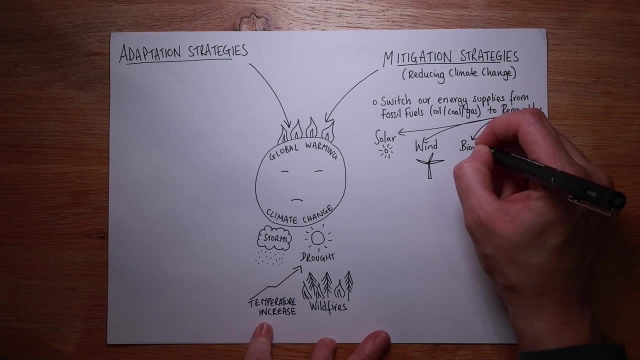 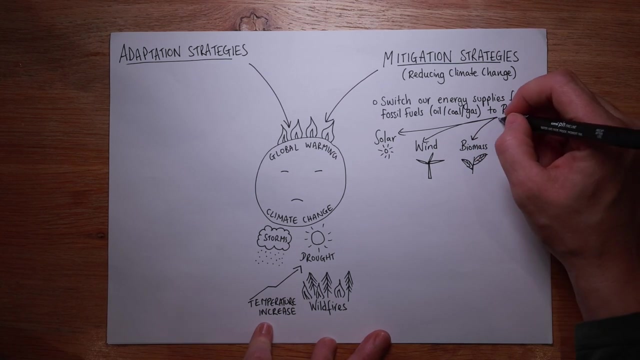 Brighton. we also have biomass which we burn to create gas. this is plant-based, so I'm just going to draw some, some leaves to remind us that, so it's working with natural materials. and we also have hydroelectric, and that can include tidal as well as inland. 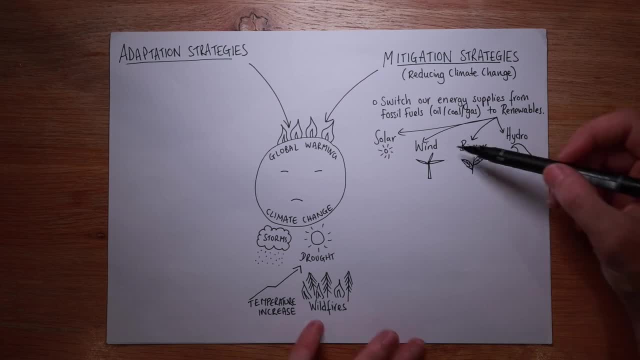 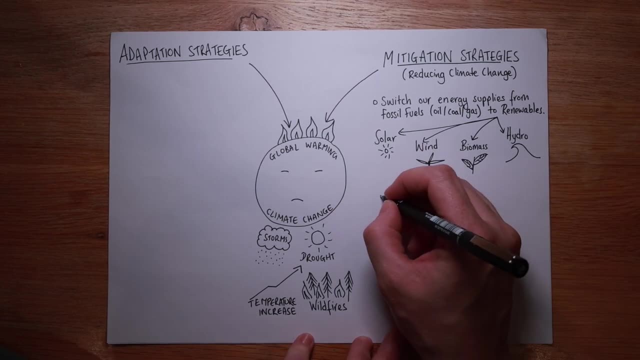 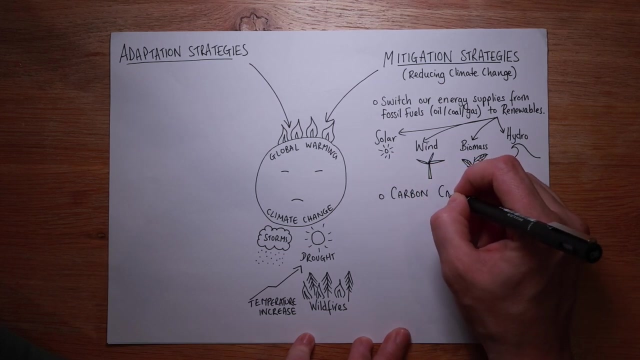 hydro, so that's from water. so we need to move to really a hundred percent renewables. unfortunately we're not there yet, right? secondly, we can do something called carbon capture. now this is relatively new. it was started in um in Iceland, and what they've done is they've actually provided all the 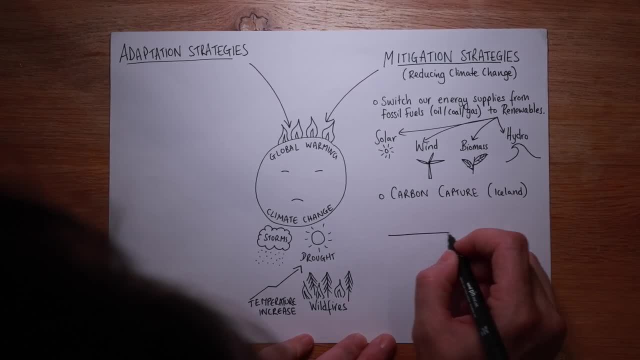 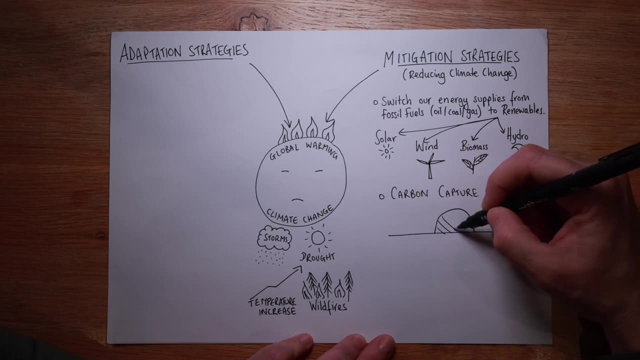 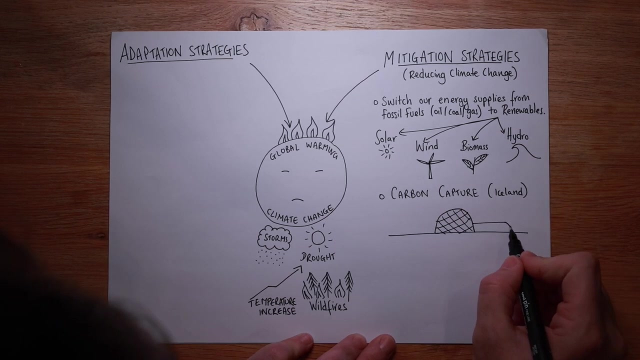 information on how to do this, basically for free, and basically encourage the rest of the world to get on board and to start making these. now. I can't really get into this in a huge way, but essentially what happens in Iceland. what they do is they suck in the co2 that's in the air and then they put it into a 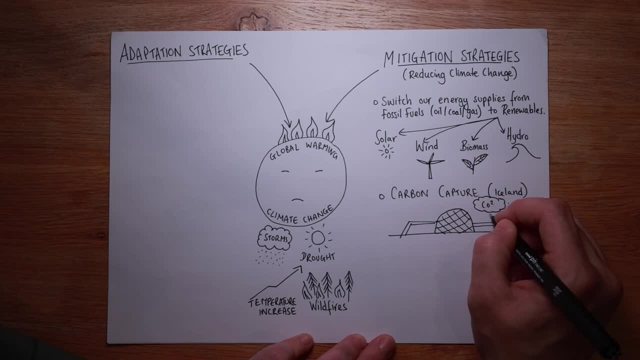 container which is, you know, in all of our atmosphere, and basically that co2 is then sent down. it goes down about two kilometers into the ground and then it is essentially calcified, it becomes rock. so after two years it kind of becomes a sort of calcium rock. 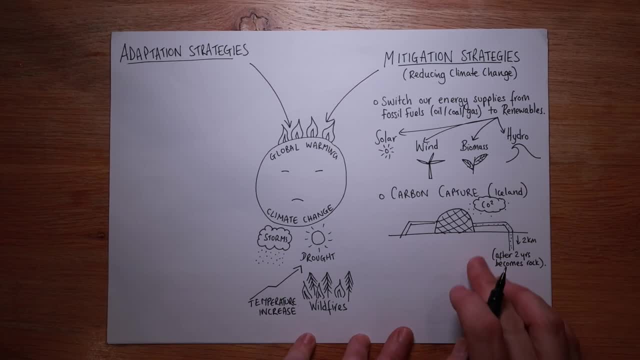 okay, that's not the best, but it gives you a bit of an idea of what goes on and, like I said, they've provided that for free. and then, lastly, I know there's other. there's the electric vehicles, as walking and cycling, but as a big one one, I guess. 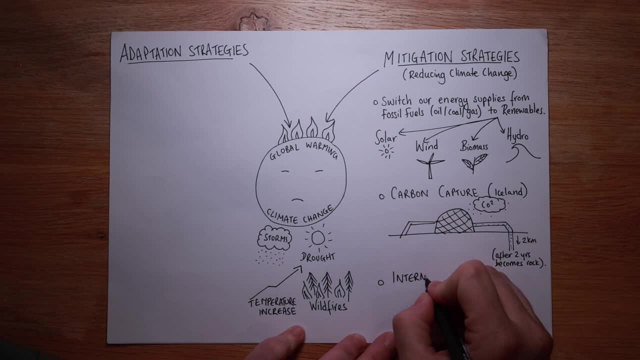 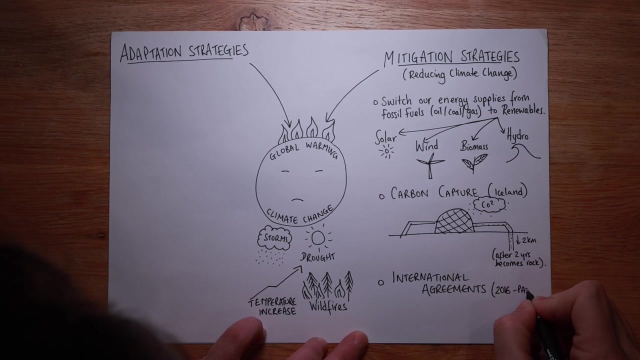 I would encourage you to use in an exam is international agreements. international agreements now we, we- we have recently had a huge summit in in Glasgow and that was part of the cop26 program, but the big ones that last happened is the 2016 one in Paris, and 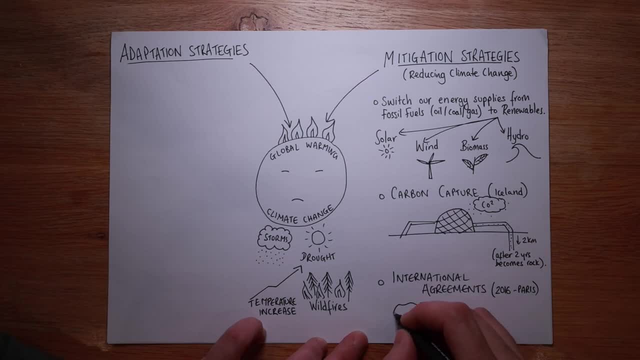 there will be another one soon, but essentially this is where countries around the world- these are countries, not clouds- get together. the world's largest leaders get together from the biggest nations- you know the united nations present and others- and they, they all, travel to one country and they meet and they agree to lower emissions. that's the. 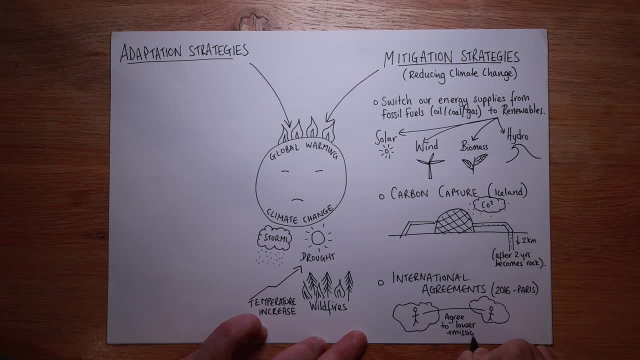 main thing that comes out of this, and the one that came out of 20 of 2016 in paris, was that we would be carbon neutral by 2050. we're not there yet, but it's also not 2050, so we're on our way. but these 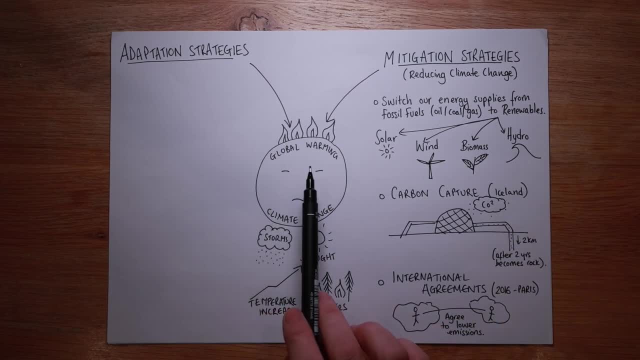 these mitigation strategies will literally change what's going on with the earth. they will reduce global warming because we won't be emitting so much emissions from fossil fuels. we will be pulling in the fossil, the co2 that's in the atmosphere, therefore not contributing to the greenhouse. 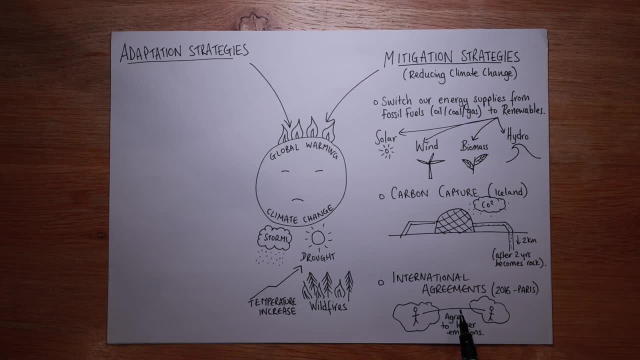 effect, and by creating these international agreements, we won't be a- you know- making things worse in the future. but global warming's here, climate change is here and we've got to deal with that in a way that protects people and their property. so let's go through some. 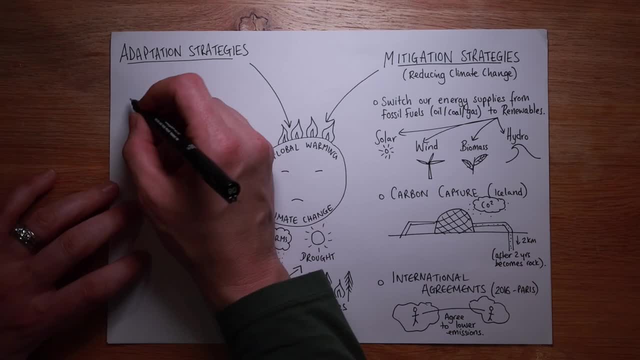 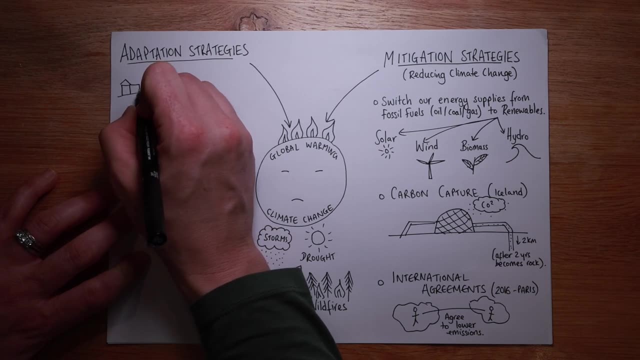 of our adaptation strategies. right for the first one: if you just draw a line and put land- and we know it's land, because i'm going to draw some really basic houses that look a little bit like beach huts- i agree. um and then, um and then. 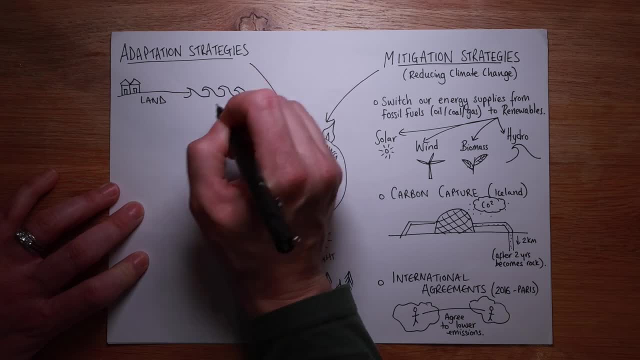 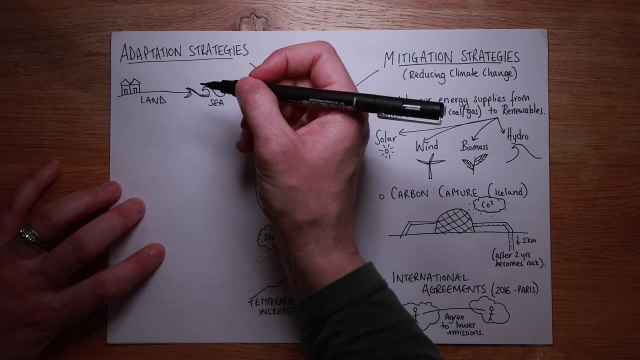 let's have some waves, not great waves, but there we go um, and obviously this is to represent the sea, but also to represent a storm surge, which we're starting to see more of in these extreme weather events. now what you can do as a as your first adaptation strategy is: you can draw on. 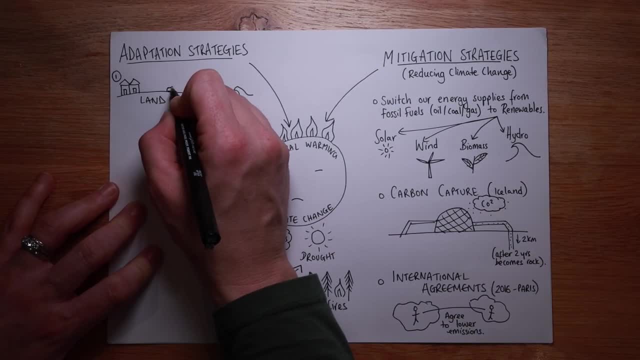 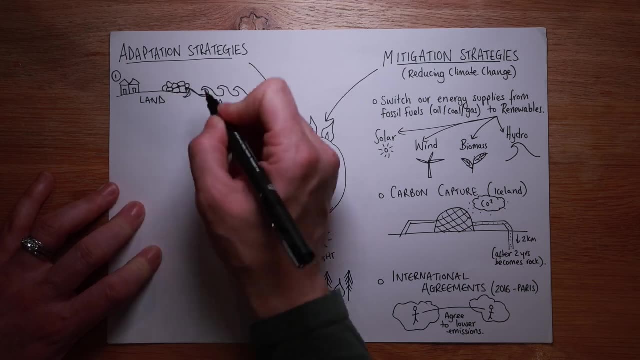 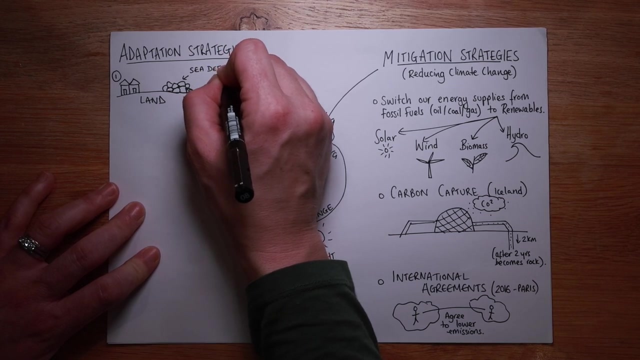 sorry, let's level that back. you can draw on some rock armor, so just some jagged lumps of granite or rock which can be placed on the beach. so i'm drawing a little arrow, i'm going to write sea defenses, and the one i've drawn here is rock armor. of course there are others. 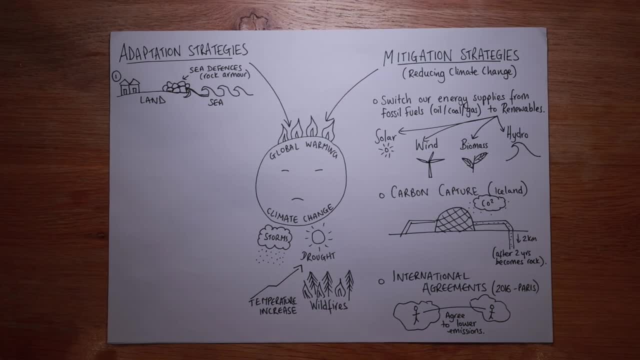 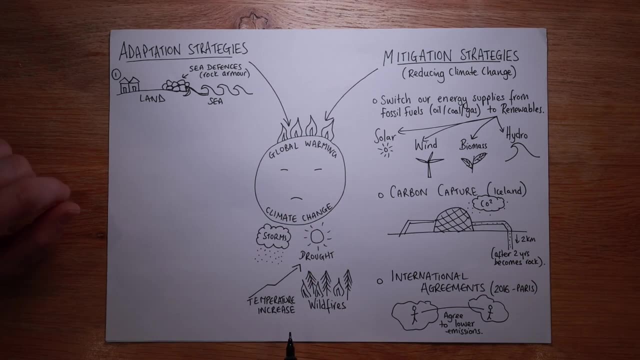 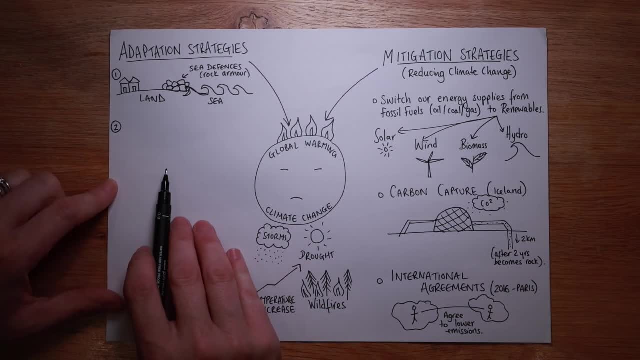 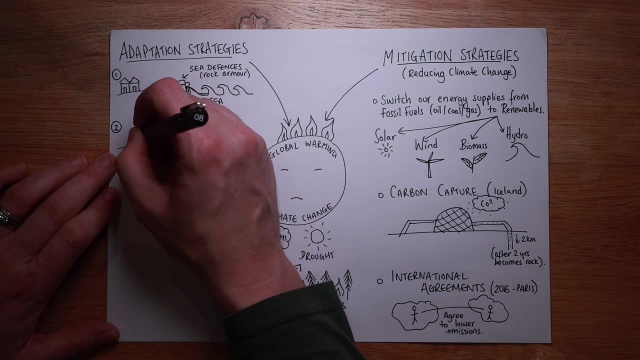 it won't last forever, but it's going to help people adapt to a changing climate. for the second one, again we're going to draw some land, and this time we're going to draw some plants in real life. they'd be much closer together and they'd have a lot. 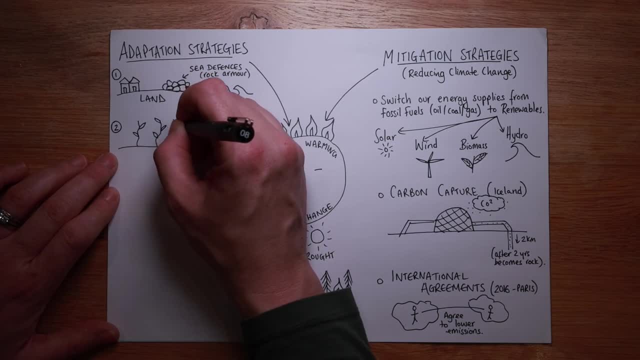 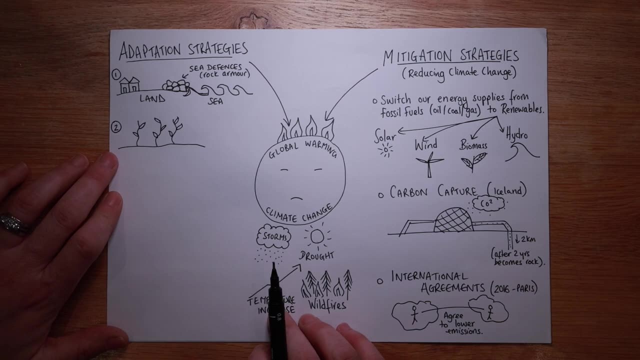 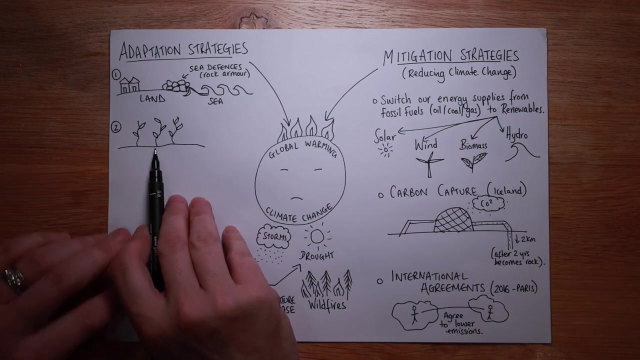 more leaves on them. but this is to look- uh, essentially to look- at farming and agriculture. we're experiencing more droughts, hotter summers and, across the world well, also cold, some cold, colder conditions as well- basically, more extreme weather. so what we need is our crops, our food. 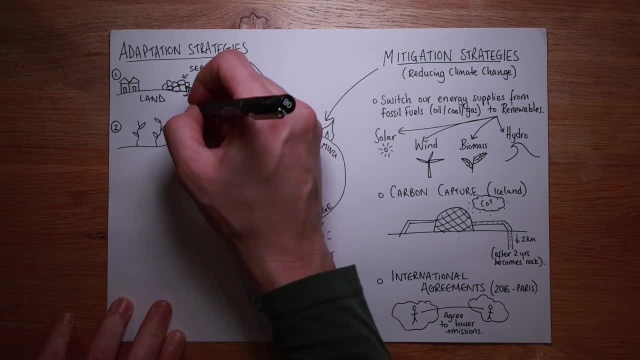 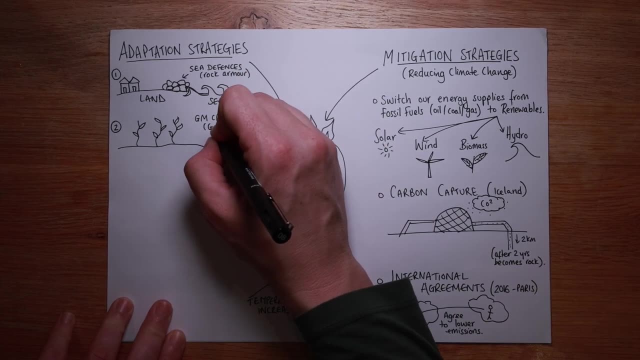 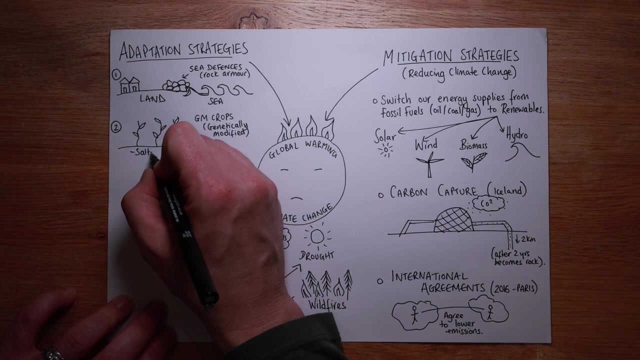 supply to be stable. so what you can do is get gm crops- gm stands for genetically modified- and you would be expected to say how they are modified. so the two ways that i want you to remember: the first one is they are salt water resistant and that means if there's a flood and 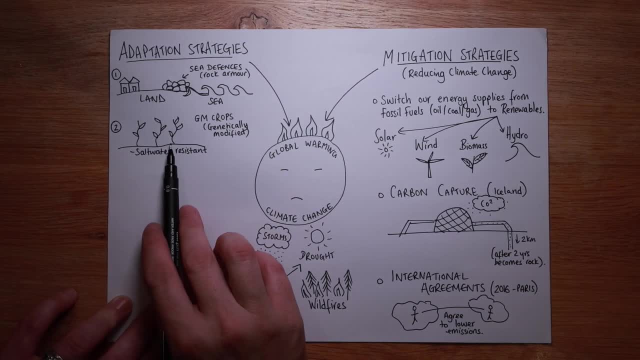 an extreme weather event and the sea floods in like as shown above, the crops won't die. okay, they can be genetically modified in a lab to be tolerant of some salt water. it doesn't mean they can be watered with salt water, it just means they will tolerate, you know, the odd flood and the other. 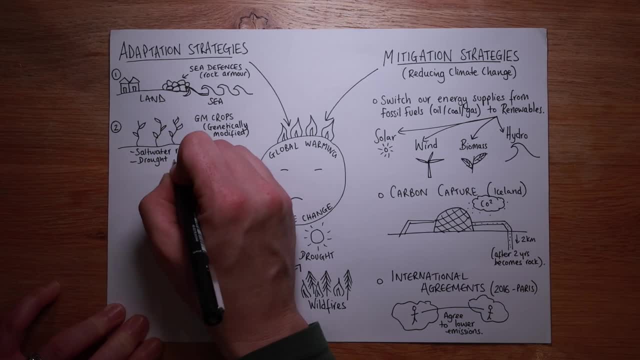 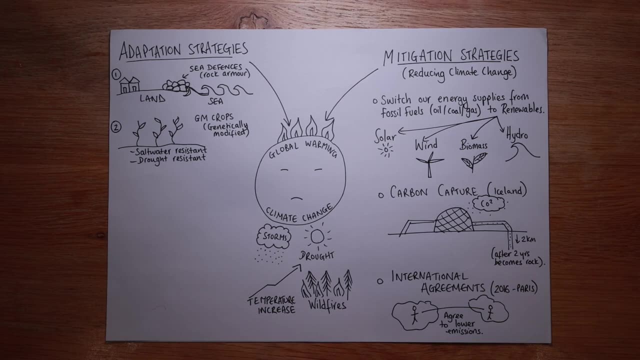 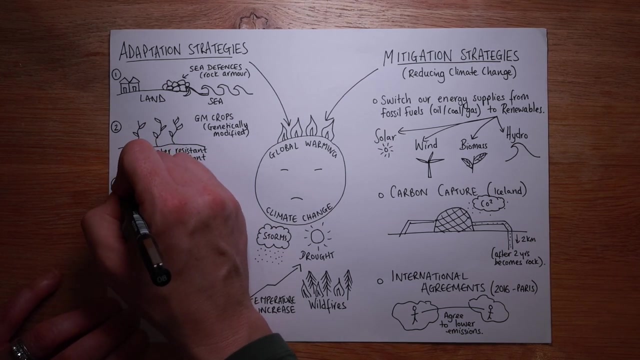 thing is they can be made more drought resistant, because water supply is very difficult and we want crops that will grow even if there isn't as much water around. okay, talking of water supply, let's make that our next one. draw a big water droplet. well, ish, big, let's have a few. well, it looks like a nose, let's. 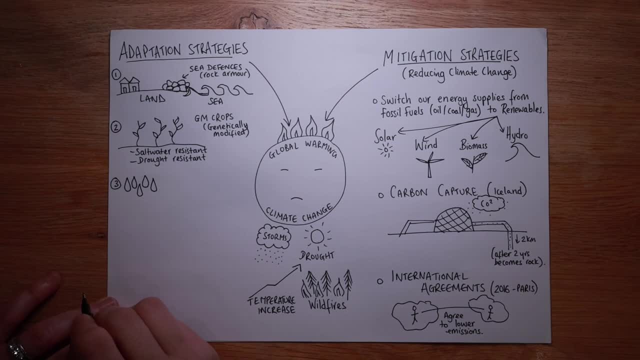 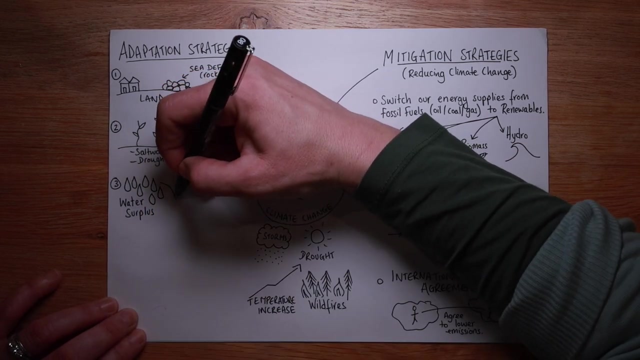 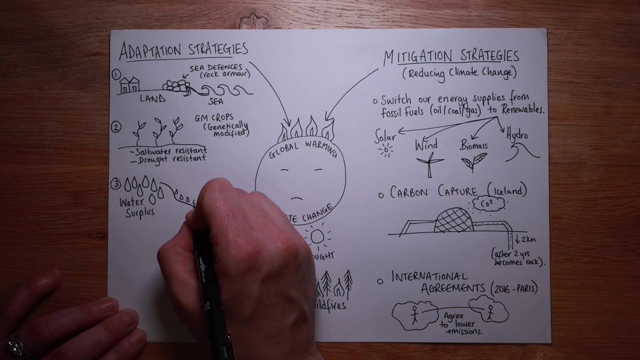 put a few more in there, we go um. so what we can do is we can move water from an area of water surplus, which basically means there's lots of water might be drawn lots of water droplets there. it can basically be moved and transported. draw little water droplets along here. okay, this is um happening in the uk at the 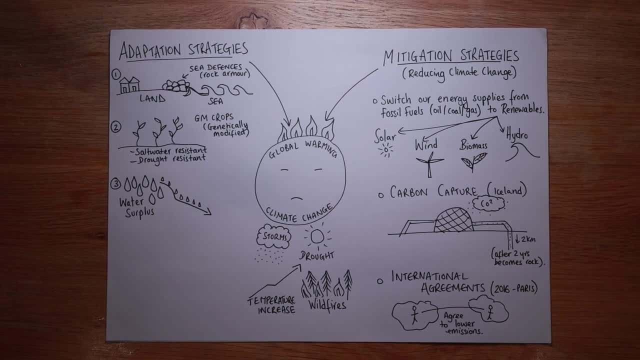 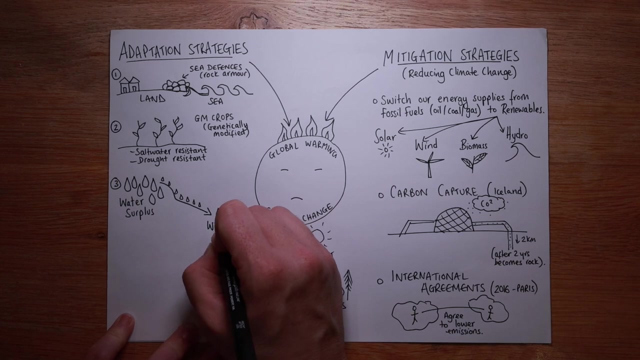 moment. so often we move water. it takes about three or four days from kilda water up in the north east england uh to the sort of london area, oxfordshire area, and we move it to an area and draw smaller water droplets, of water stress. these regions like london and the southeast are areas that have very 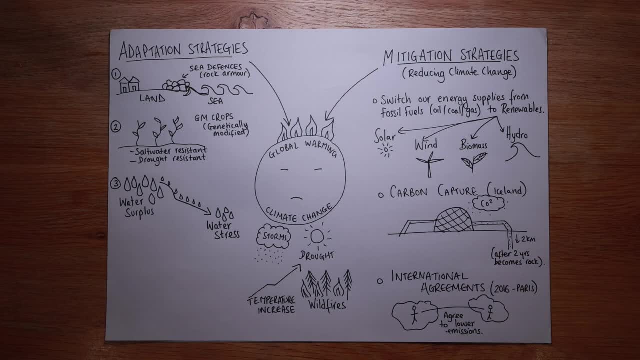 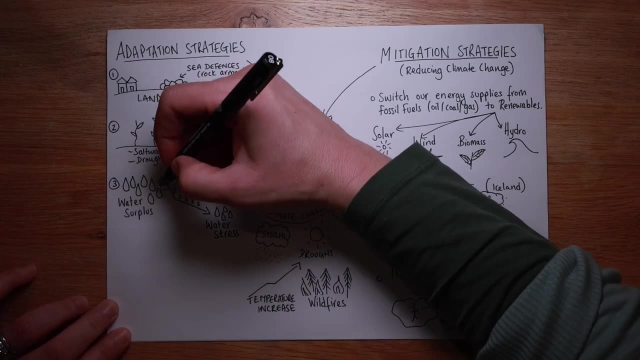 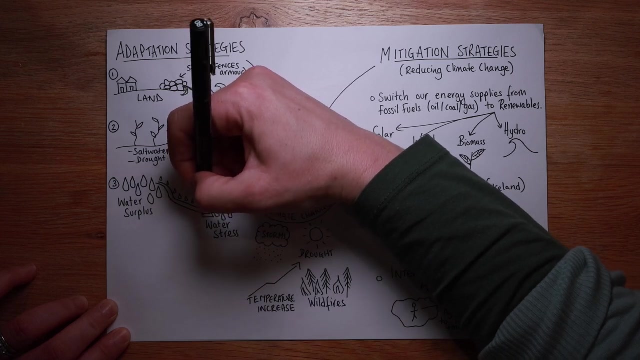 little water, very little rainfall, essentially, and offered in high populations. so we're going to see more of this for climate change. so we might have to look- i'm just going to make that up bit bigger- we're going to have to look at more ways to basically get this water moved. 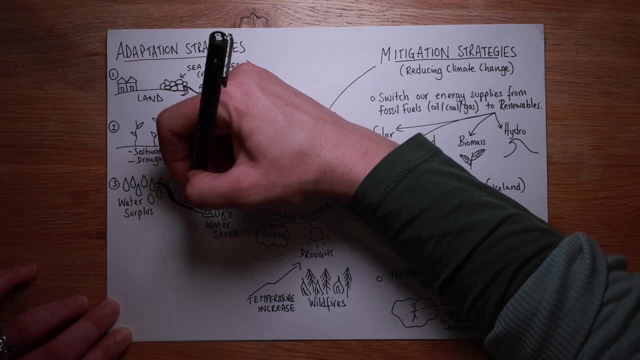 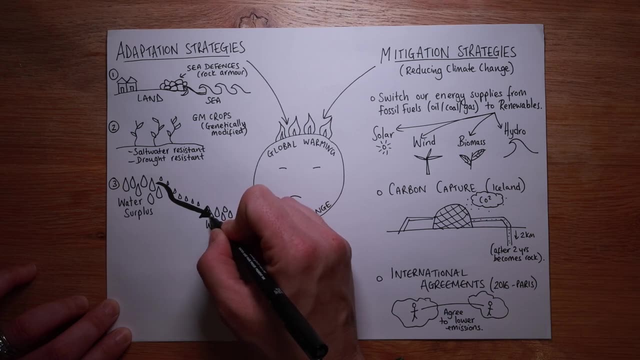 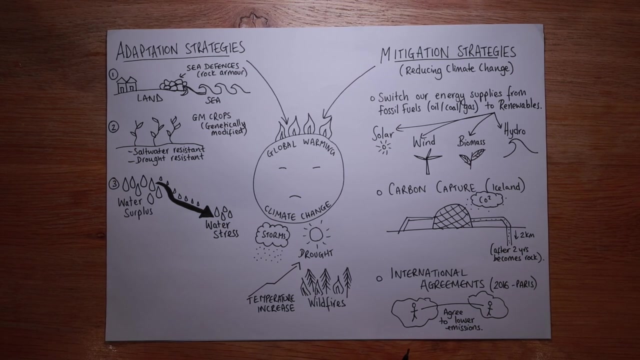 i'm just going to draw it in. it takes, like i said, three to four days to pump it. it's not cheap. it does use energy, so it's not like an absolutely amazing situation to be in, but water is essential. okay, right, last one, and it's such a classic i know we talked about 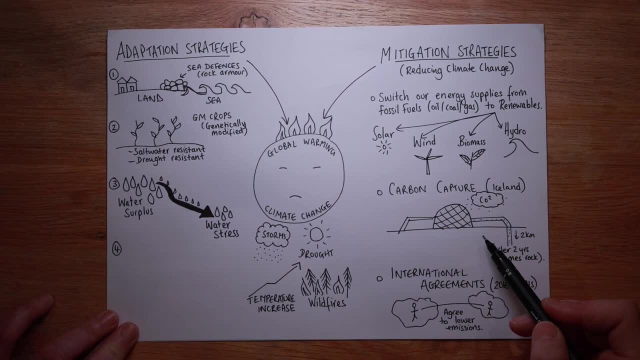 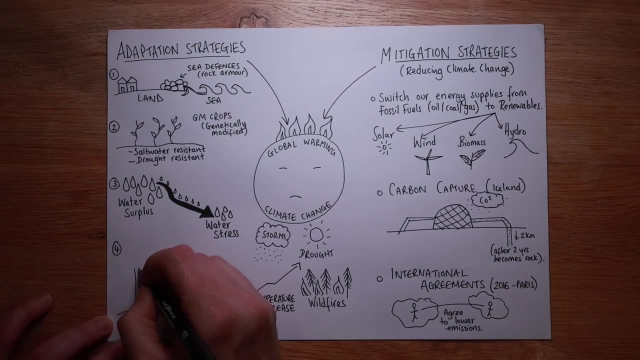 carbon capture earlier, and that being a really good mitigation strategy. but this one is so natural and it does it all on its own, and these are trees. so just draw a tree, exactly like you would have done at primary school. really doesn't matter what kind of tree you draw, let's have lots. 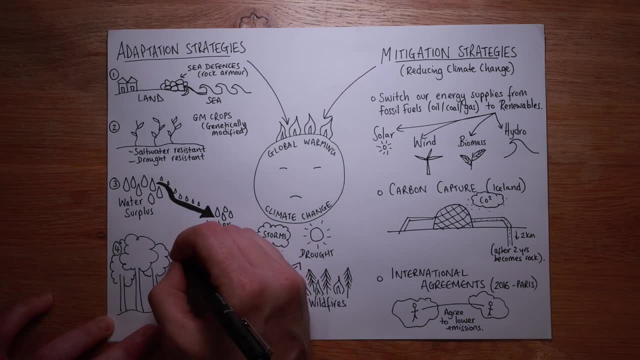 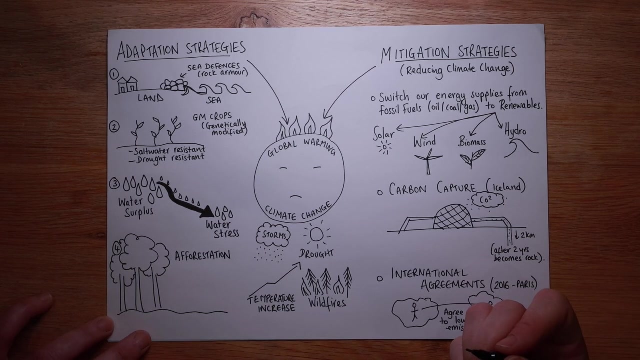 of trees. absolutely love trees. now, this is cool. the proper word for this is afforestation. i'm going to put that in capitals: afforestation. now, that is the opposite of deforestation, so it is basically planting trees. trees naturally do what carbon capture does with huge amounts of technology.